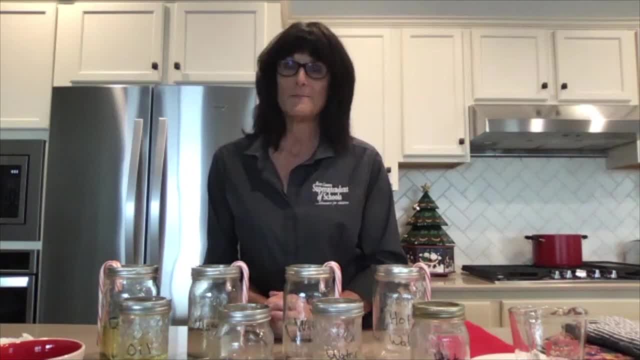 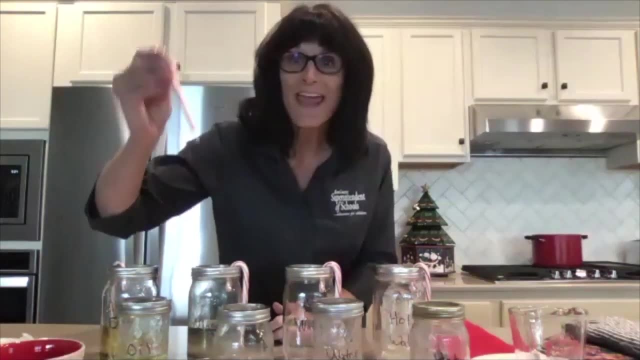 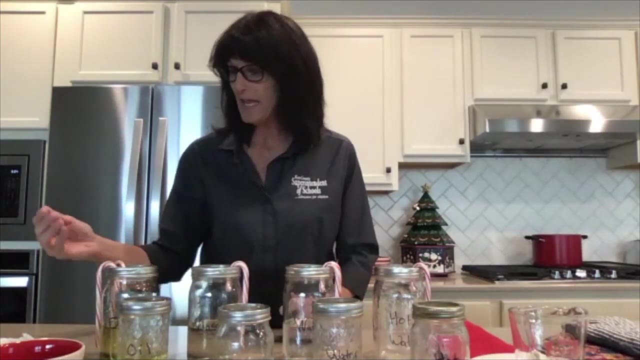 I thought it would be fitting for us to do a holiday themed science experiment. And who doesn't love candy canes? So today, for today's experiment, I call it very simply: Dissolve Candy Canes. And for today I have some large candy canes. 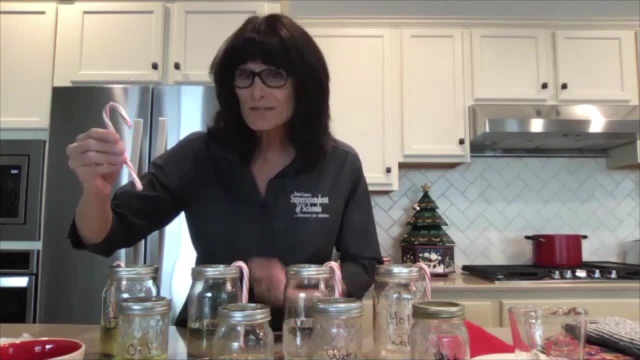 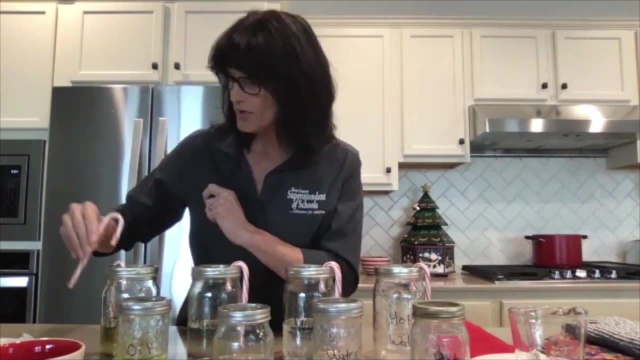 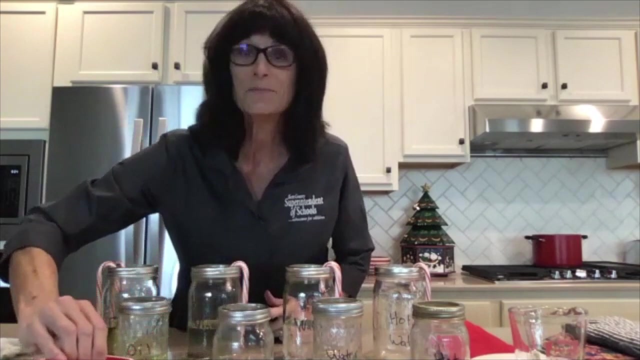 And you might find that it's a little difficult to unwrap these large candy canes without breaking them. If you break them, that's fine. It's just important that you have that larger ratio of candy cane. for our experiment today, I also have some smaller candy canes. Oops, I spilled those on my table. 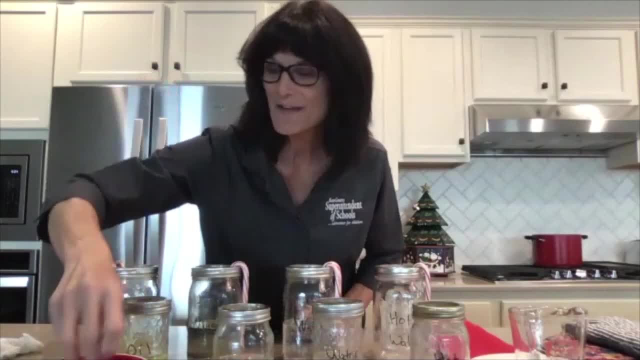 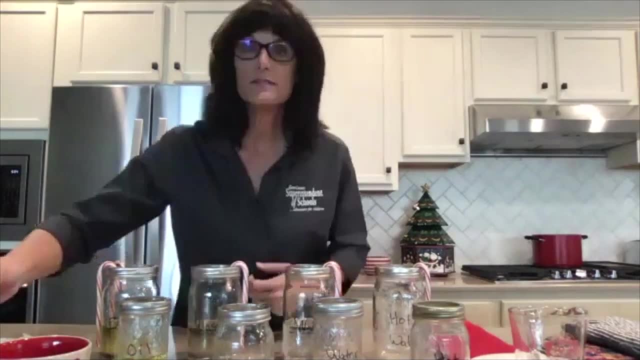 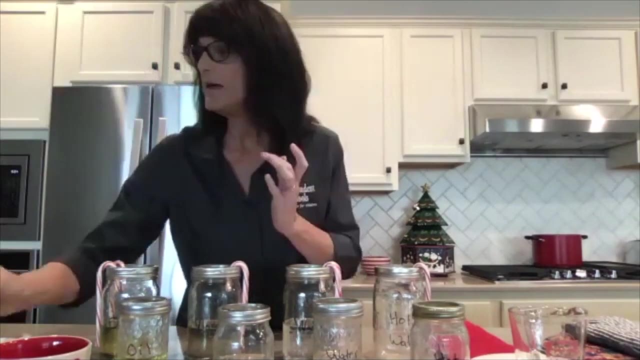 I've got some smaller ones for you as well. We'll be testing them. We're testing some small candy canes versus large candy canes. We also have some oil, just vegetable oil. Any kind of vegetable oil from your kitchen will work. 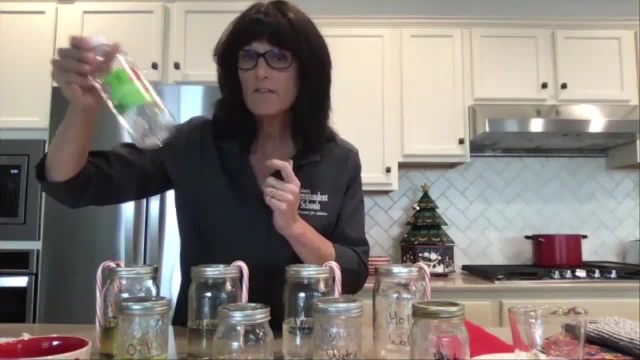 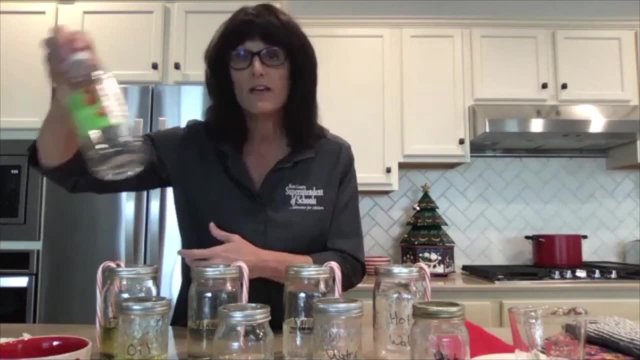 I also have some vinegar and any kind of vinegar- white vinegar from your kitchen will work, And actually it might be kind of fun to. if you have apple cider vinegar or any other kind of vinegar that you have in your kitchen would work as well. 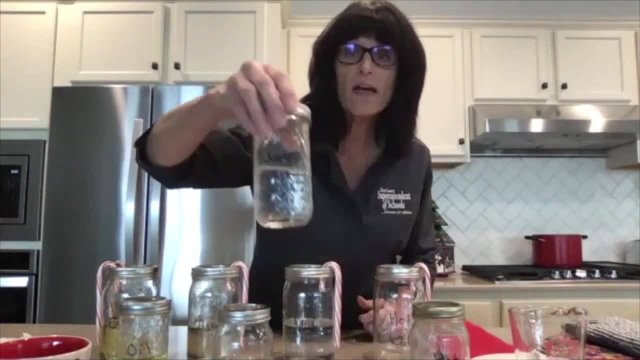 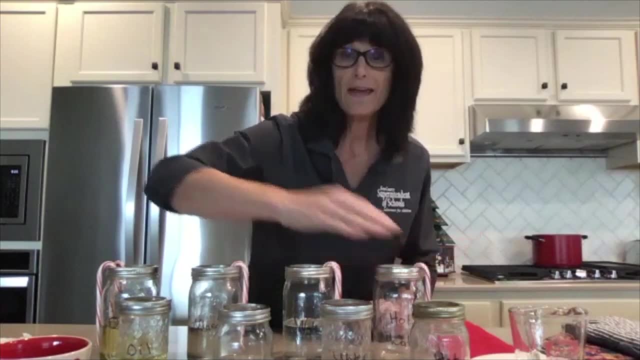 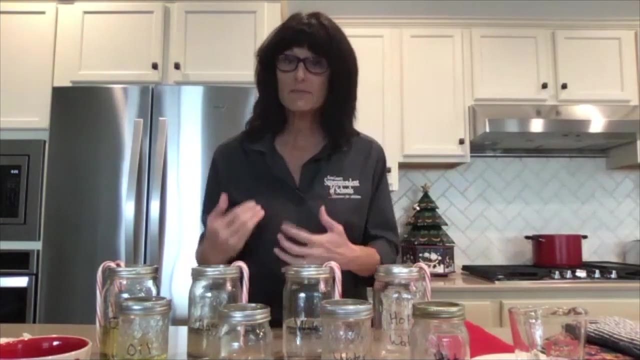 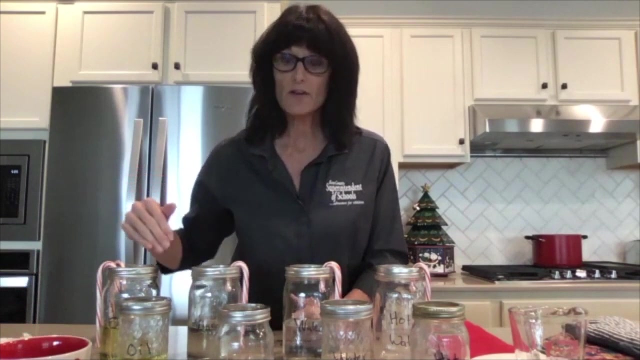 We're just looking for different sorts of liquids. I also have in my container already some tap water- just regular tap water- to go, And I also have back on the stove back here some hot water ready to go for our experiment. So once we get rolling, here we will be for today's activity, testing small candy canes and large candy canes just to check out what happens when we put them in our different assortment of oil. 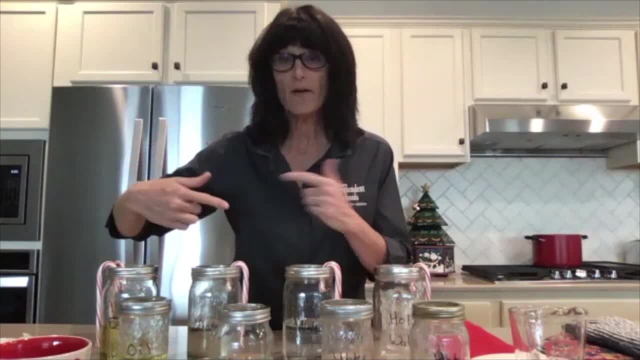 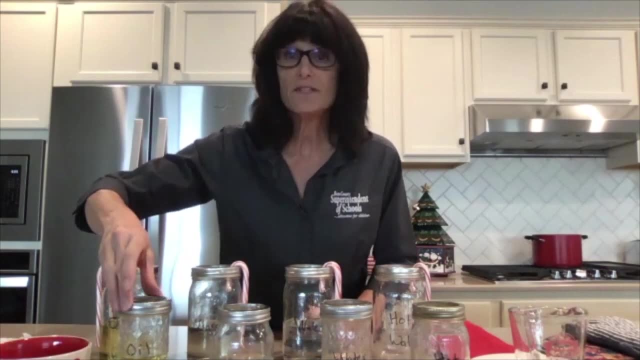 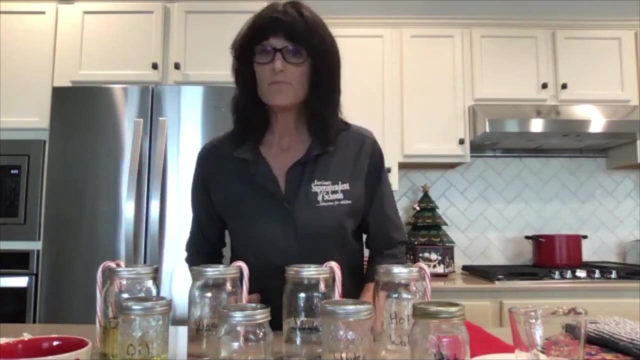 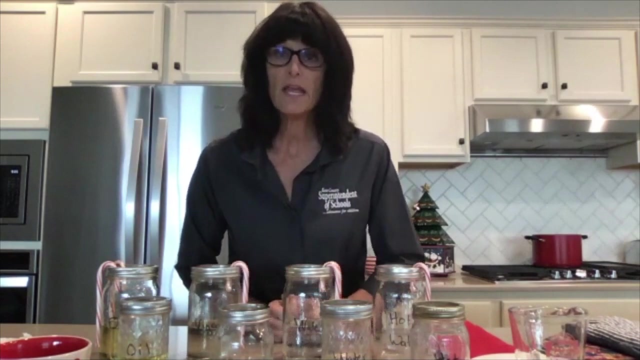 And just compare. either. we'll be comparing things like the rate of dissolving or just how the different items react in the liquids. For you at home, if you want to use a timer when you drop your candy canes in, that would also be great as well. 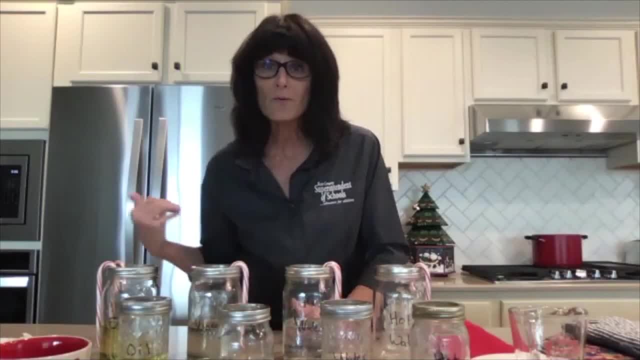 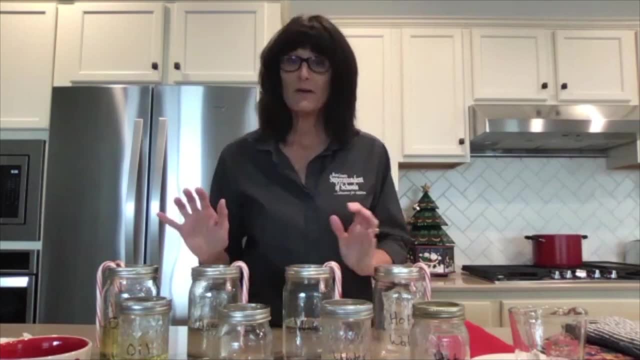 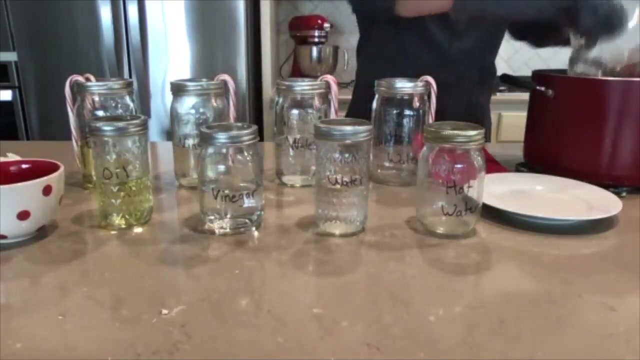 So if you have a cell phone timer or a timer in the microwave, like I do back in my kitchen, either way would work. So that's how our experiment is going to work. So as we add our hot water, I do have some warm water here. 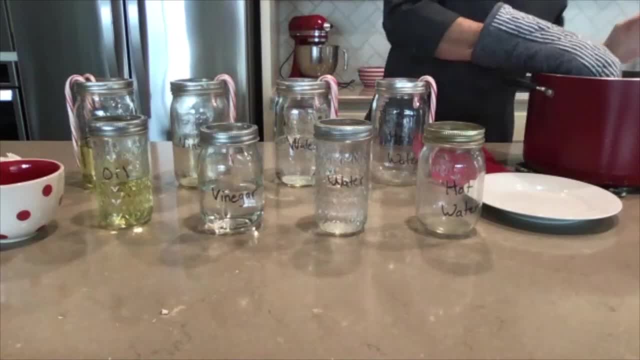 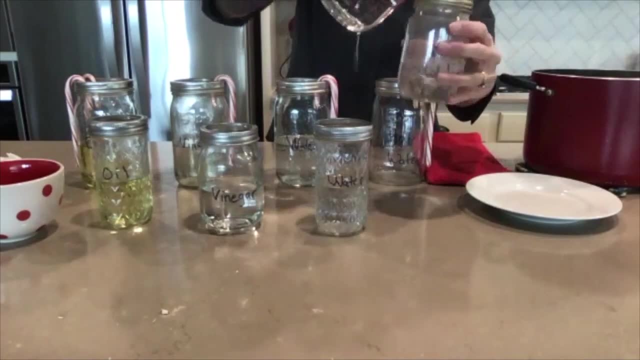 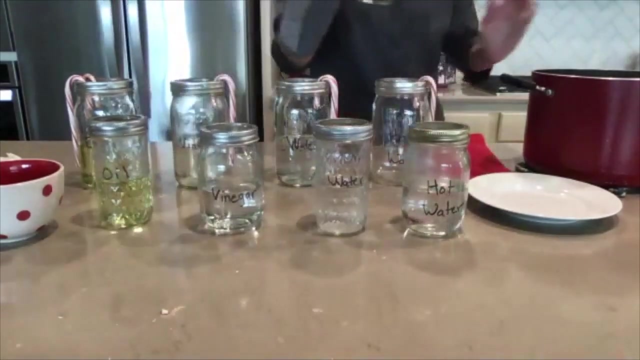 And you'll notice that I have my trusty dusty pot holder on. This is definitely a part that you'll need a grown-up to help you with. I need to pour some hot water into my container- About the same amount as the liquid right next door. 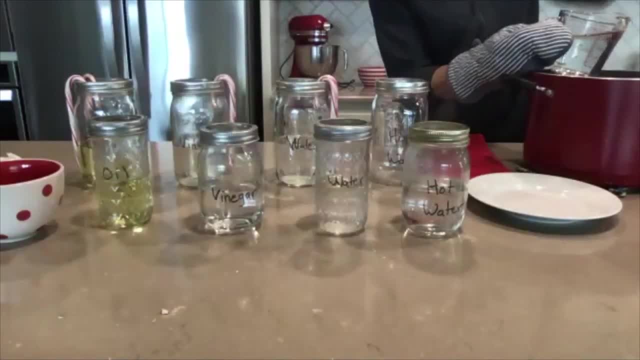 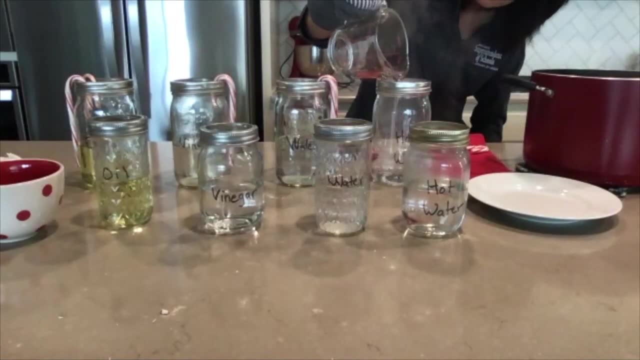 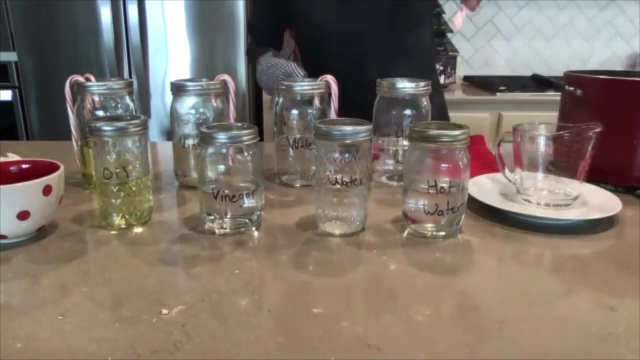 And then I'll add some hot water to my larger container And back about the same amount as the container next door. Let's see just a little tad more of my hot water. That looks about the same. So my other large candy cane ready there. 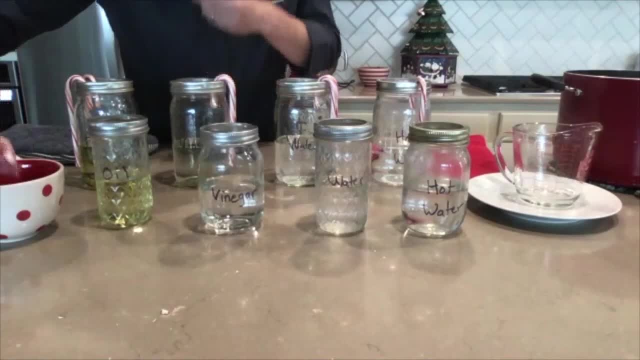 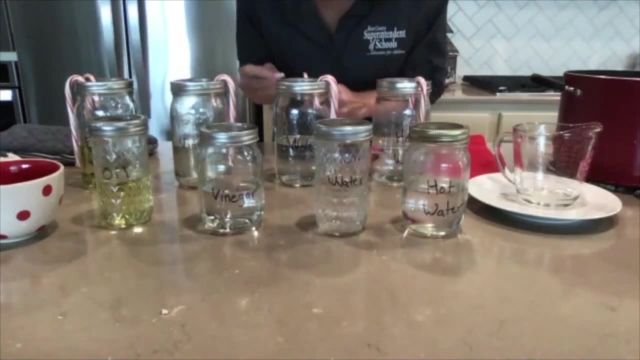 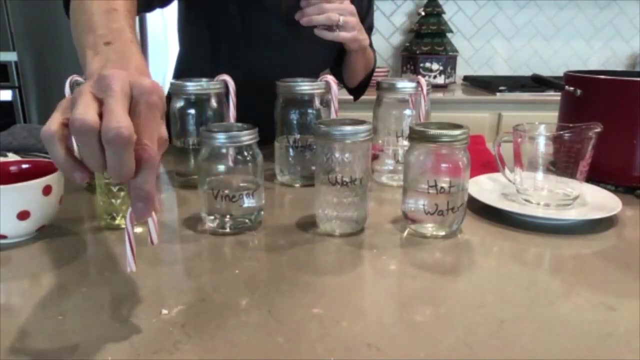 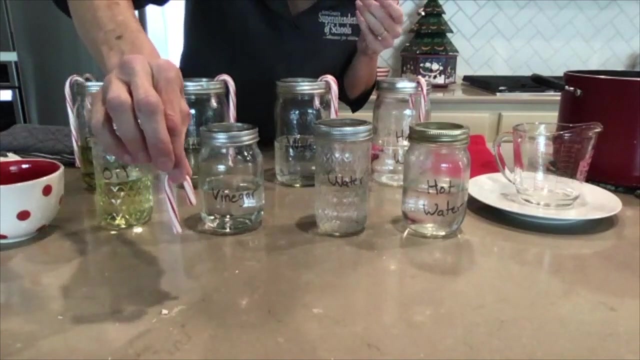 All right. So what I'm going to do is go ahead and do my experiment, And what I'm going to test first is how the small candy cane, how it reacts. Just do some observations around reactions, Not going to get too specific about timing the reaction. 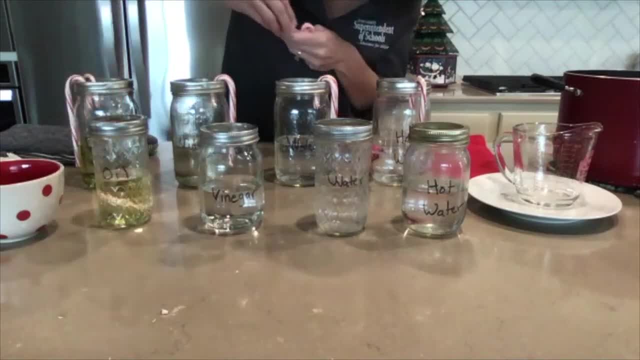 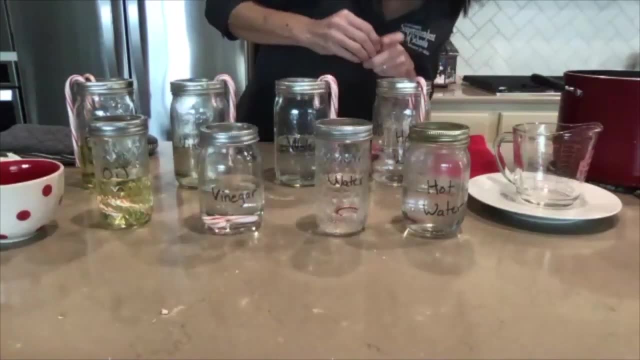 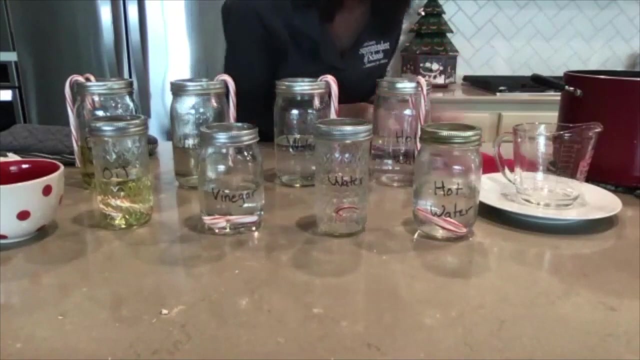 So my small candy canes in the vegetable oil, in the vinegar, in the room temperature water and my hot water? Ooh, I'm hearing some cracking in the hot water. And see how it goes. Let that sit for a minute. 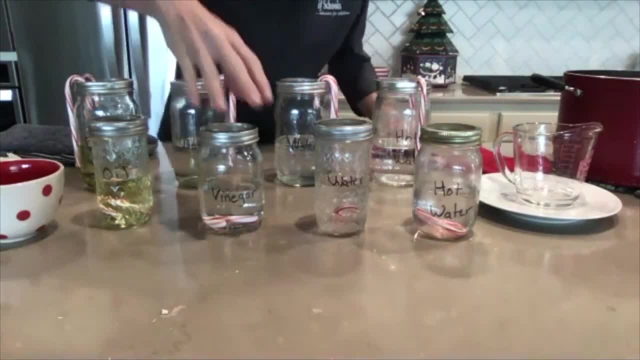 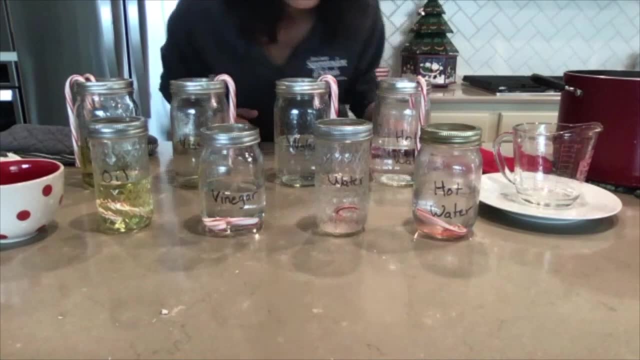 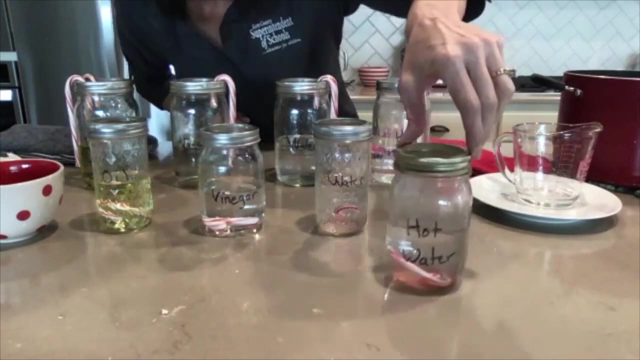 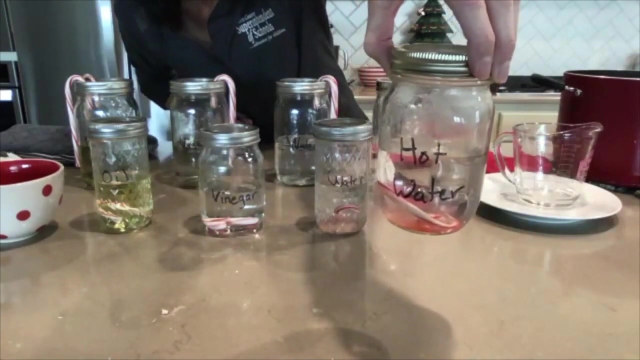 Should be starting to see some reactions. What are you noticing? I'm starting to see some bubbling in the hot water. Move that a little closer to the camera. Let's see if you can see. Oh, it stopped bubbling for a second. 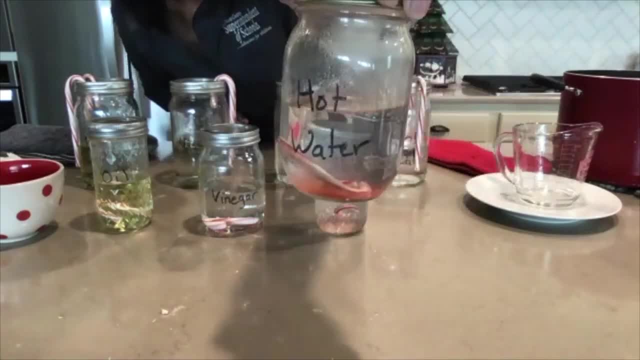 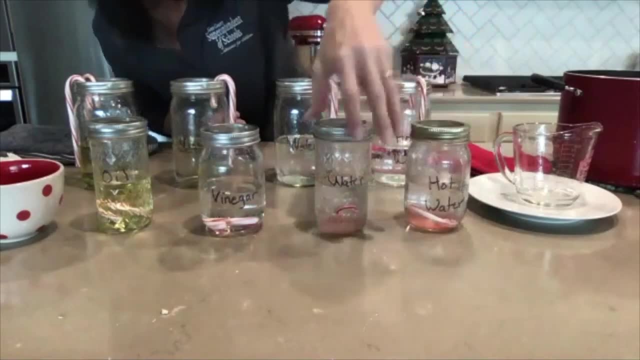 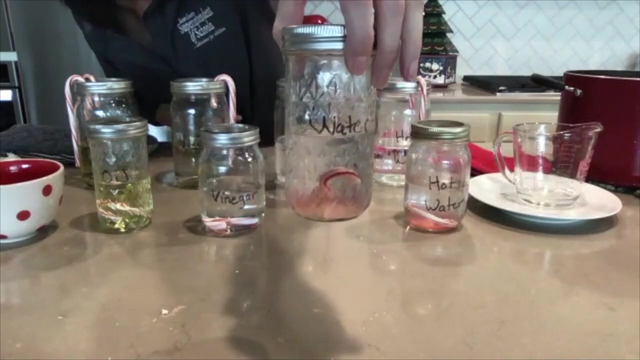 But you can already start to see some of the red color die in the hot water coming off the small candy cane. Ooh, I'm starting to see something going on. What are you observing There might be? as you're watching this play out, it'd be great to pull out your handy-dandy. 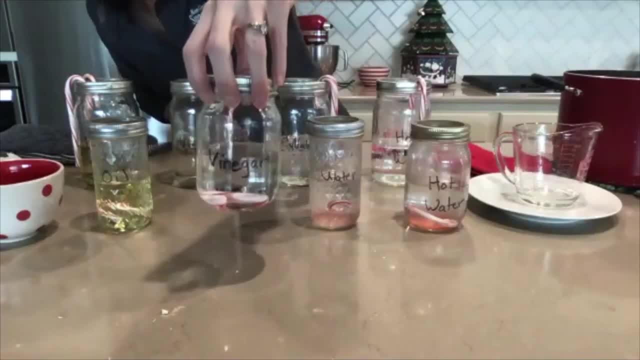 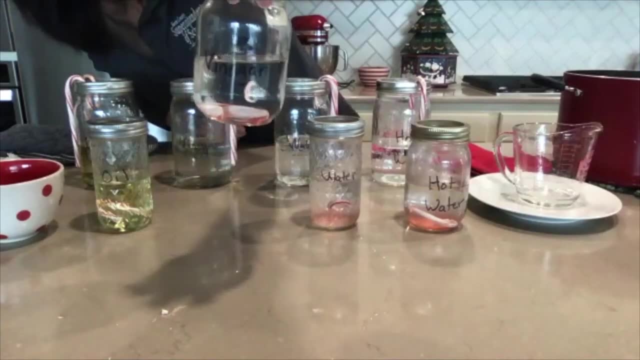 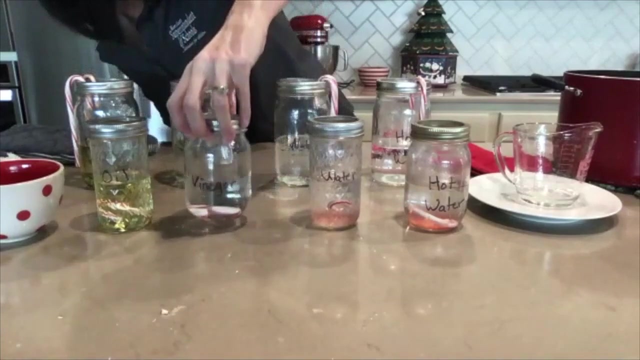 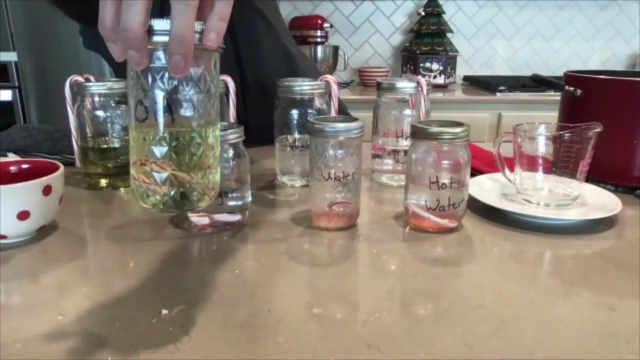 science notebook and start making some notes about observations. What are you seeing going on In the vinegar? not seeing Starting to maybe barely see some pink coming off my candy cane And my oil. I'm not observing a whole lot going on there. 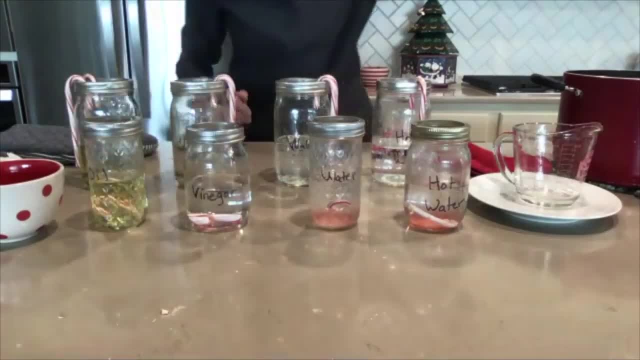 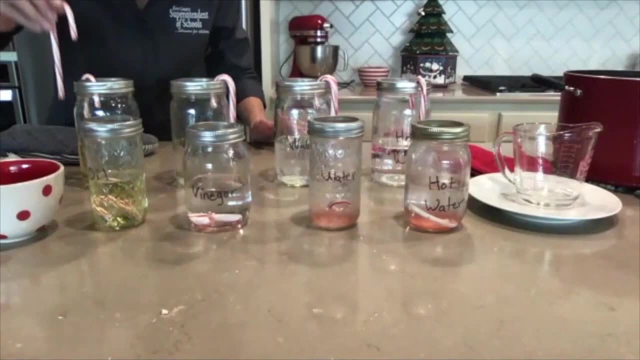 So I'm going to let those sit for a bit And while my small containers with candy canes in them are continuing to dissolve, I'll go ahead and take my larger candy cane. Probably hard to tell. See the difference. My little small baby candy cane. 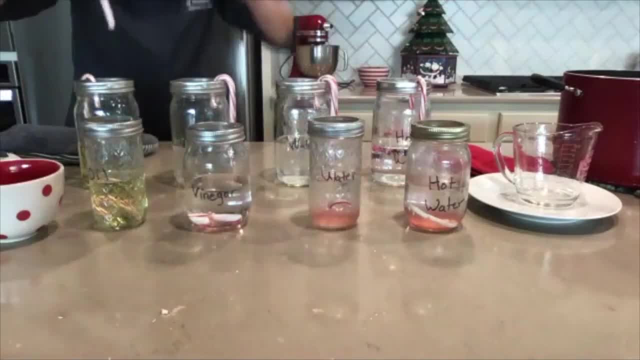 I'm going to take my large candy cane and put it in my oil- in the back I've got another big candy cane that's not broken- In my vinegar, Then in my room temperature water And into my hot water And as a scientist, I'm going to be making comparisons between lesser and higher temperature. 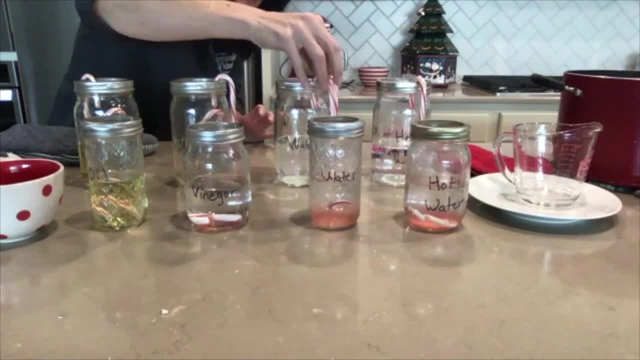 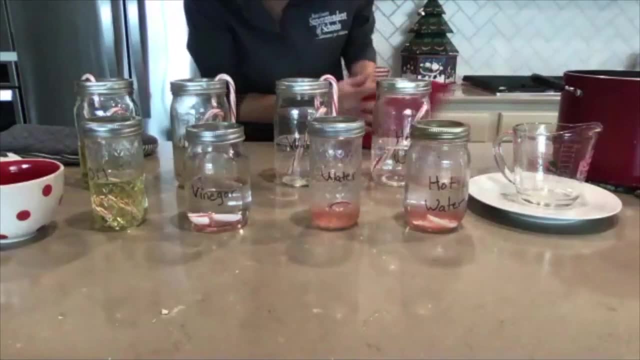 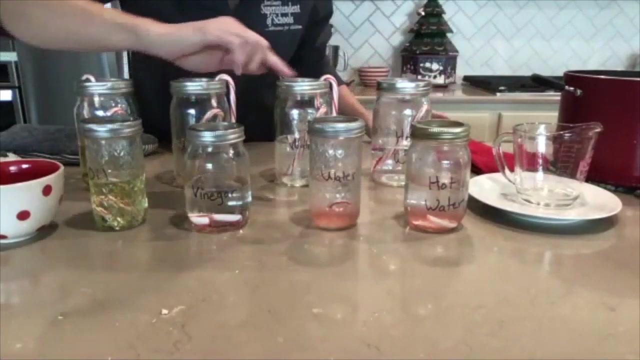 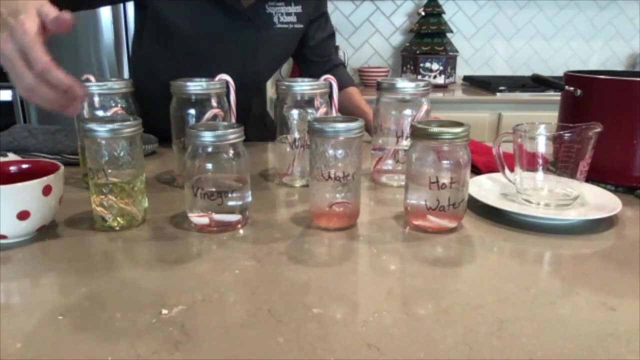 water. So I'm going to take my little baby candy cane and I'm going to put it in my hot water And, as a scientist, I'm going to be making comparisons between lesser and higher temperature water And, as I'm in a PCR test, I'm going to be taking a sample of the two in my little 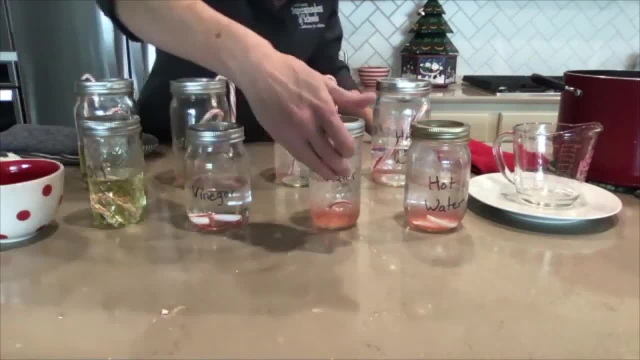 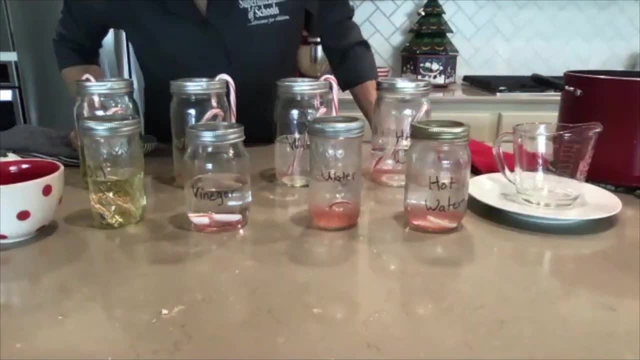 bonnecane right here And now I'm out trying to find out if they all dissolved the pink from doing some things. It just makes it so clear now And Awesome, We're back And I'm going to try to get the pink bacteria out of there. 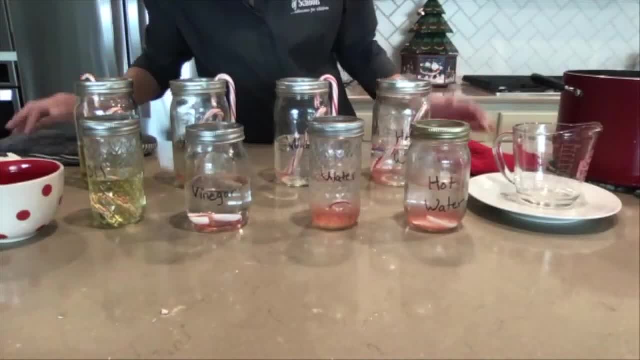 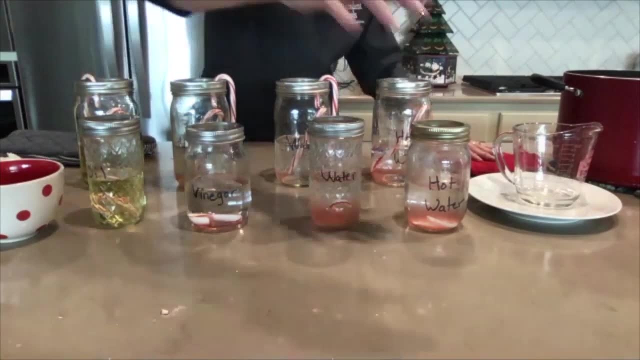 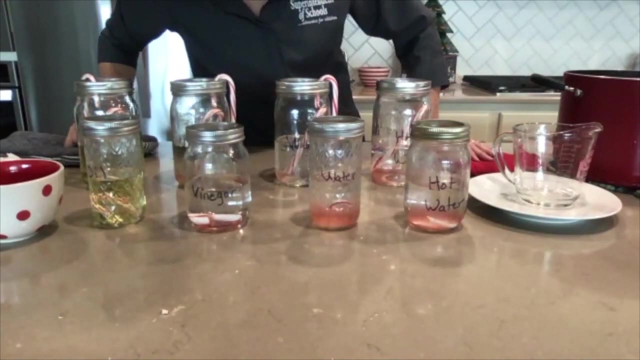 Now, All right, You're as smooth as a marble. might even consider leaving the containers out all day long and coming back and observing them periodically throughout the day. I do have to say that prior to putting my candy canes into these different liquids, 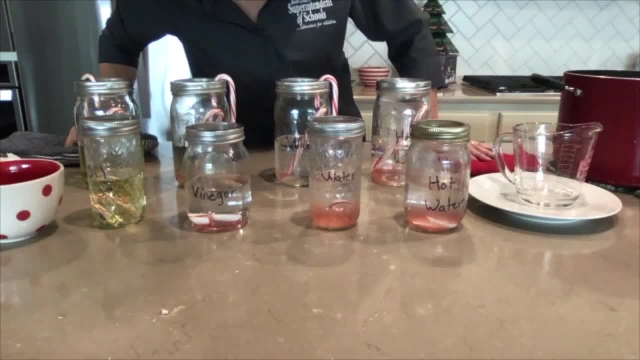 I was thinking about some predictions around what I thought might happen with our candy canes in the liquid. And you know, young scientists. I am surprised Because what I was thinking is that the vinegar- because I've noticed that vinegar seems to be kind of a stinky, strong liquid and I was predicting that the candy cane would dissolve. 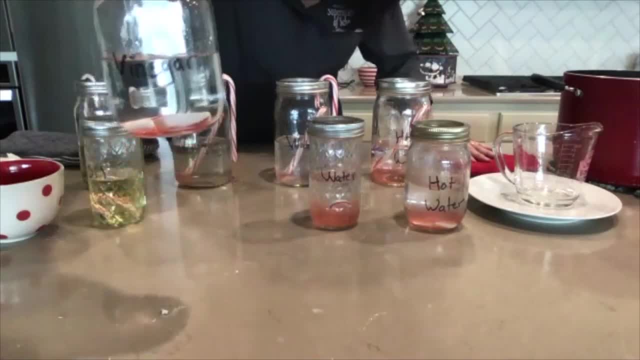 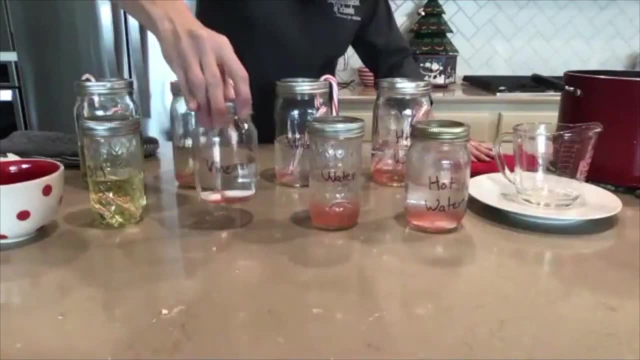 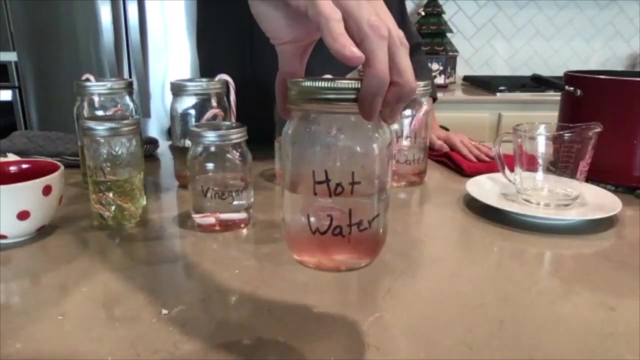 quite quickly in the vinegar And you know, I'm just barely starting to see some of the red start to come off of my candy cane. But it's the hot water where I'm really seeing a difference in the dissolving of the candy cane. 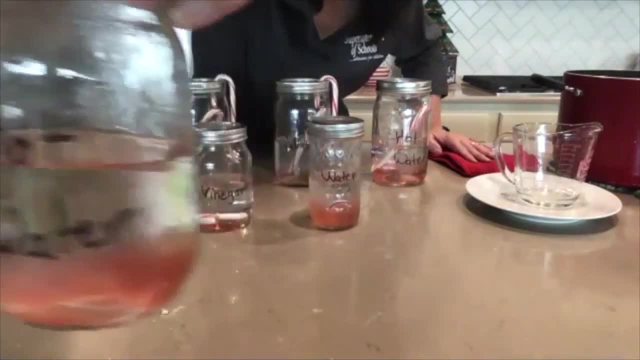 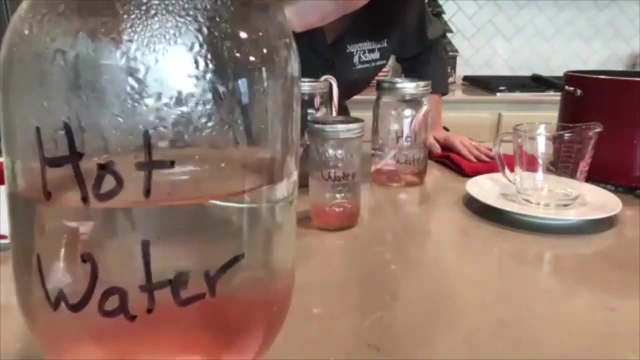 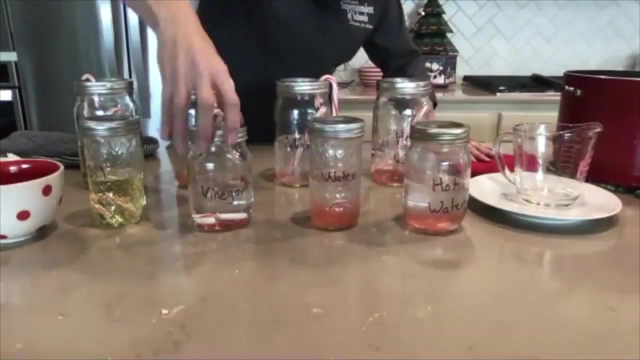 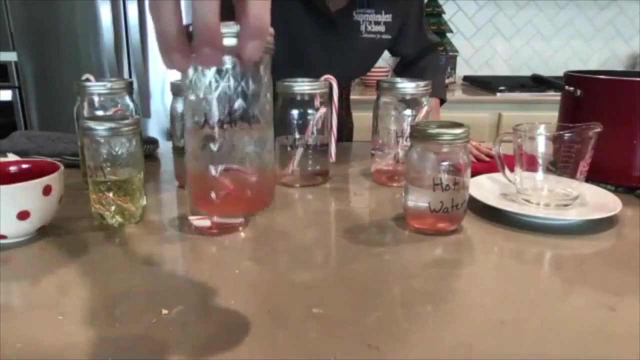 And actually I can get it even closer. oops, the candy cane has actually broken in half and there's no color left at all with the hot water, My vinegar candy cane- not a whole lot exciting going on there. It looks like in second place in terms of rate of dissolving is the room temperature. 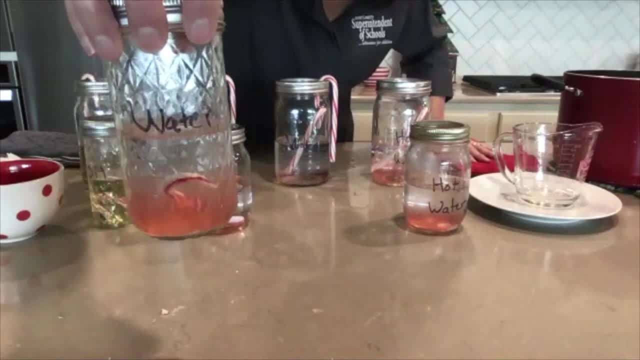 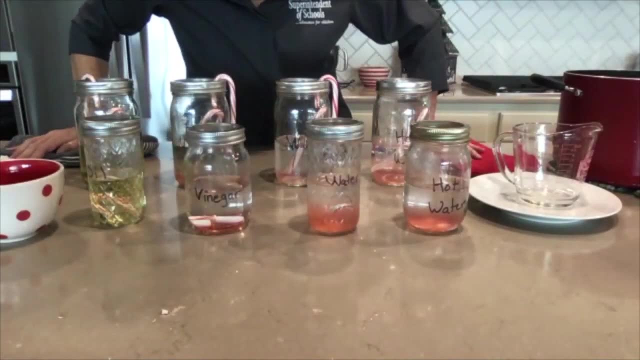 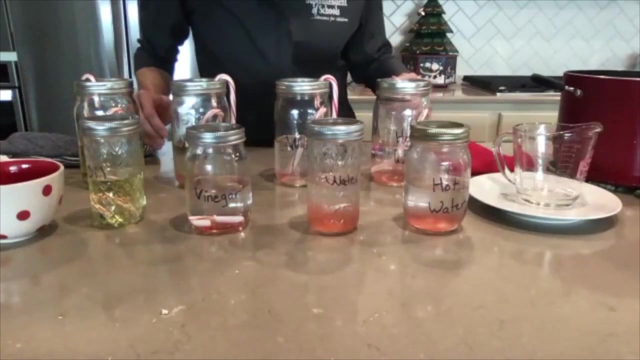 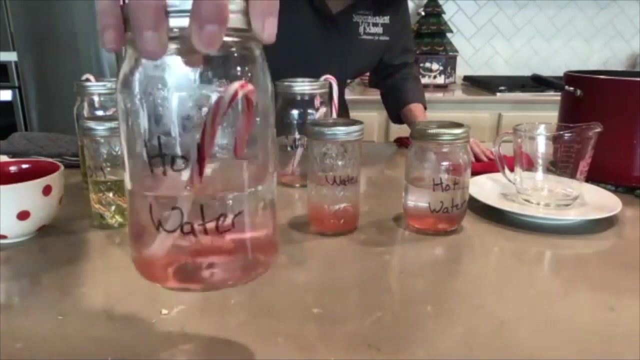 water, So my prediction was not correct. my experiment today proved my initial prediction was not right And as I'm looking at my back row, I'm noticing that I'm getting the same results That my large hot water container with my large candy cane in it. it's the same thing. 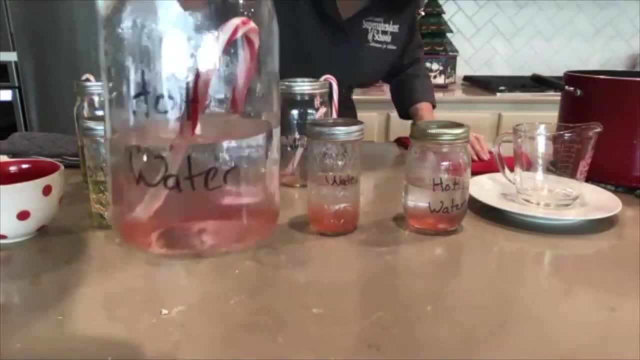 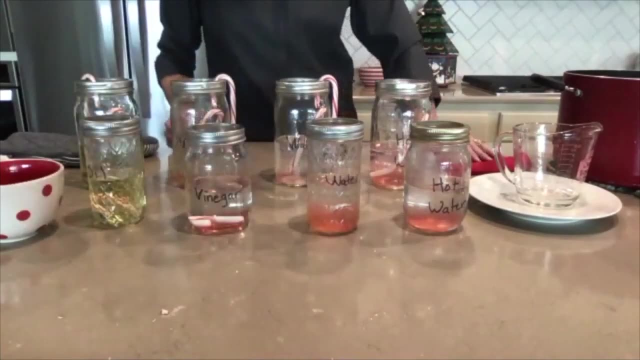 is happening. The candy cane is dissolving much faster. You can see that all the color- the red color in the hot water, is gone in my hot water. Everything else is consistent with what we're seeing going on with the smaller container. So we have lots to learn about science in our kitchen, as well as lots to learn about. 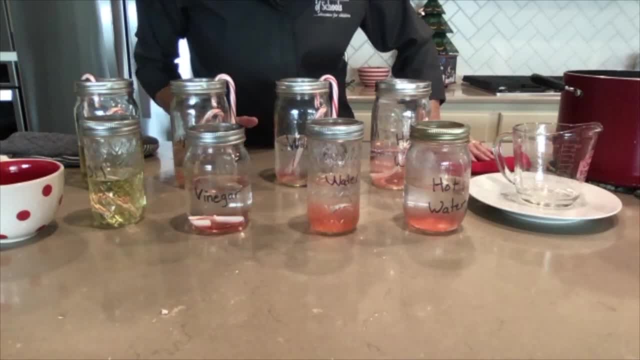 science around holiday items. So I hope you enjoyed doing some science in your kitchen. I hope you enjoyed doing some science in your kitchen. I hope you enjoyed doing some science in your kitchen. I hope you enjoyed doing some science with me this morning. I sure had fun doing science with you.